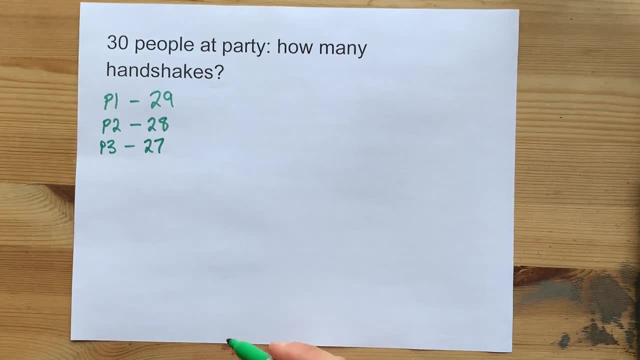 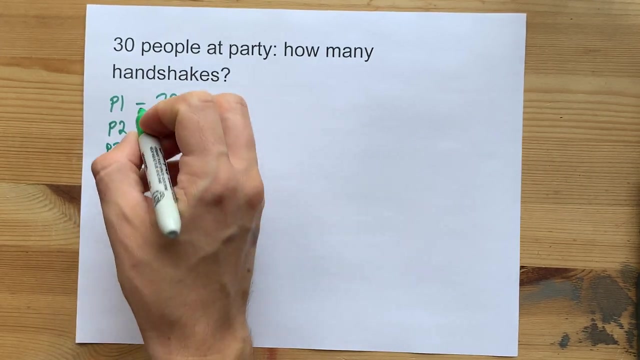 needs 27 more handshakes because they're not going to do it with themselves. We've already counted Their handshake with person one and person two. You can probably already see the pattern here. We need 30 people And the number of handshakes that are remaining to be done by. 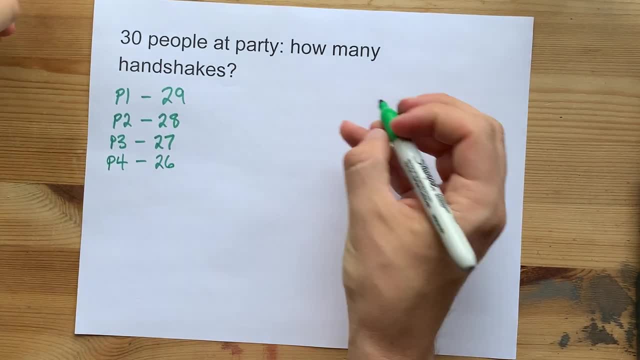 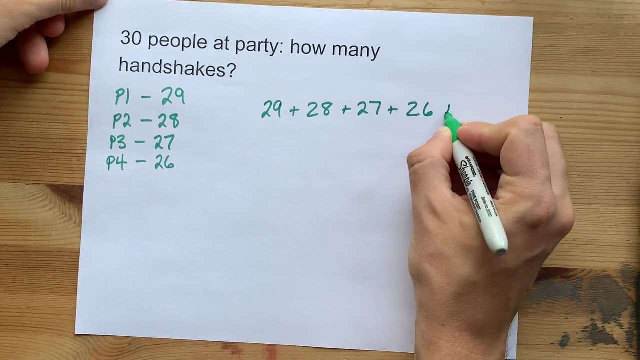 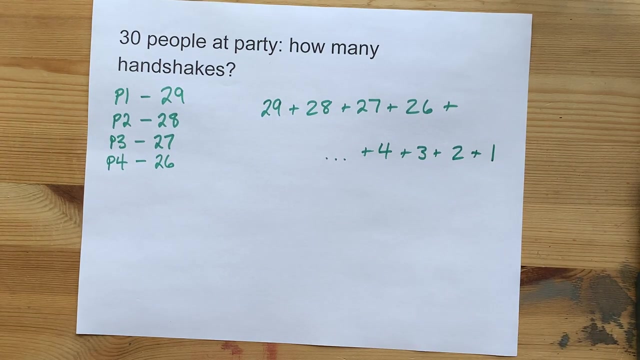 each successive person is going to lower each time. So what we have here is 29 plus 28 plus 27 plus 26,, all the way down to plus. So we're going to have 24 and three and two and the one final handshake, Cool Shall, we do. 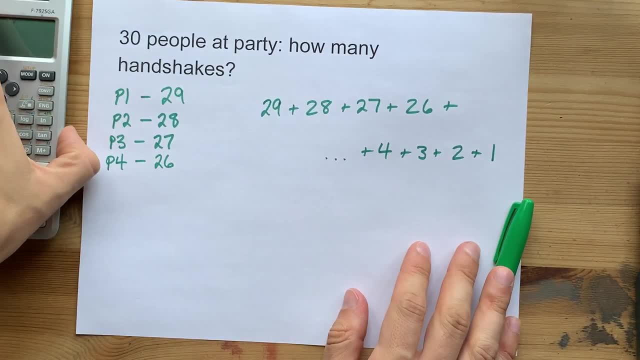 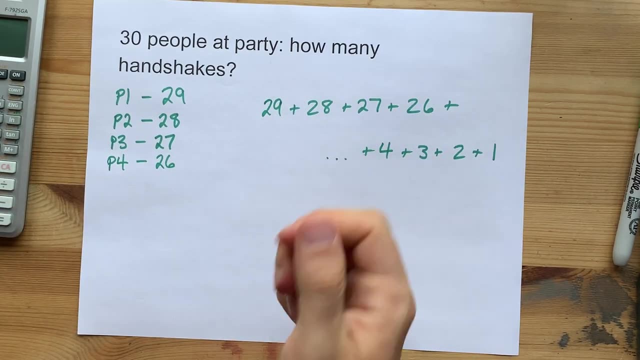 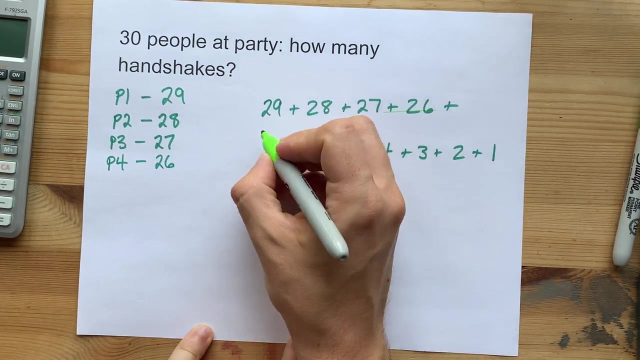 that on our calculator together. That actually sounds really annoying. I don't think I want to type it all all at once. Boy, I wish there was a shortcut. Well, there are two shortcuts. First, what you might notice if you were adding up all these numbers together: 29 and one add to. 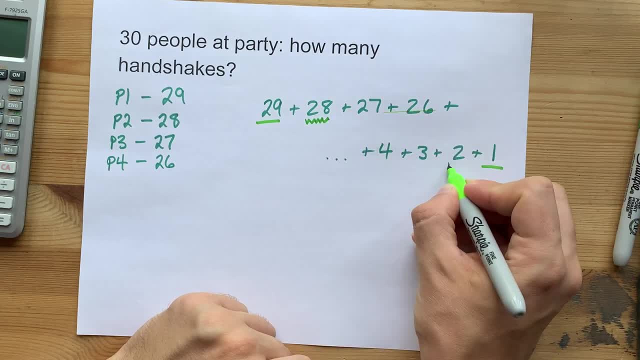 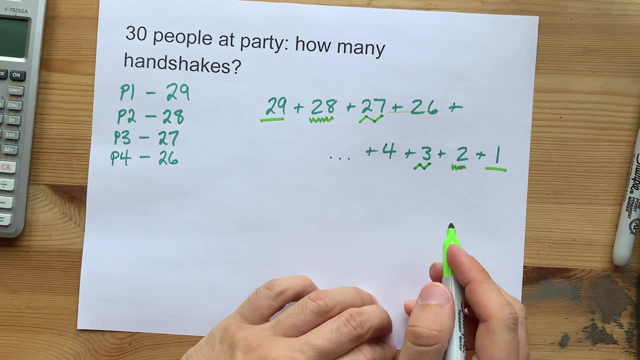 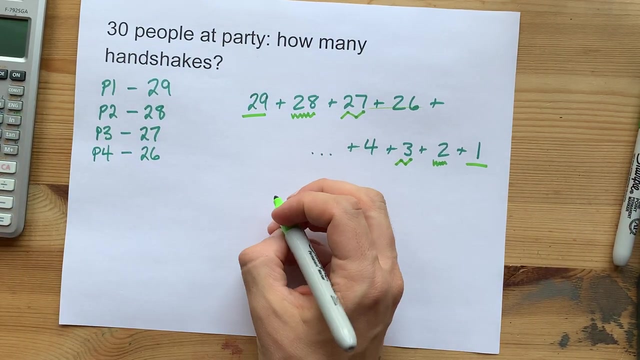 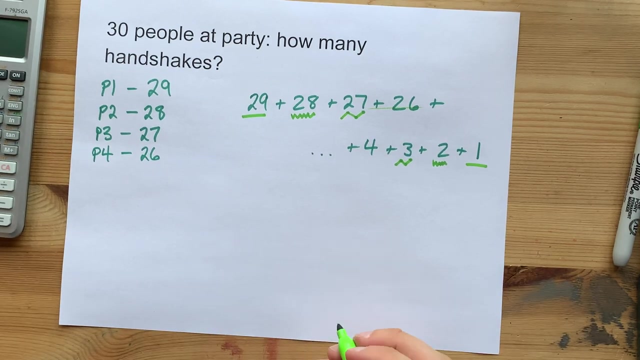 30.. 28 and two add to 30.. 27 and three add to 30. So you can keep creating pairs that add to 30 as long as you work your way into the middle. here The question is, how many pairs of numbers are there? We started at one, We got up to 29.. So 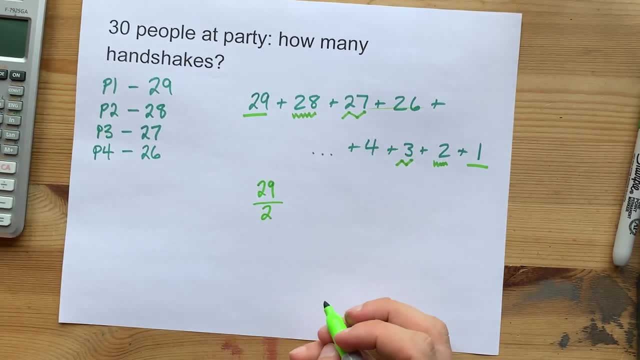 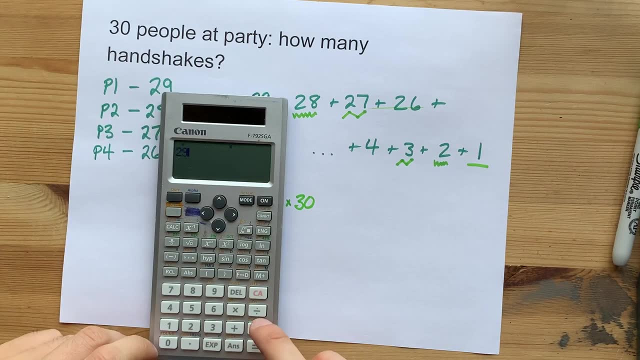 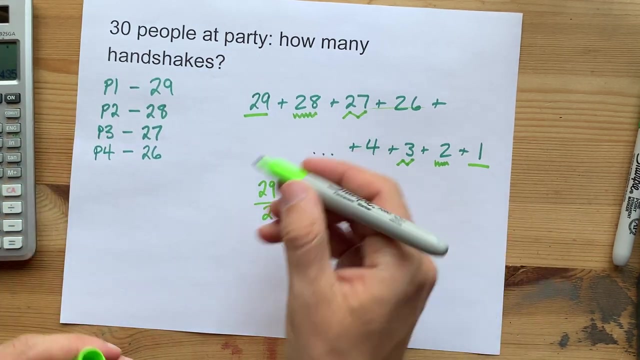 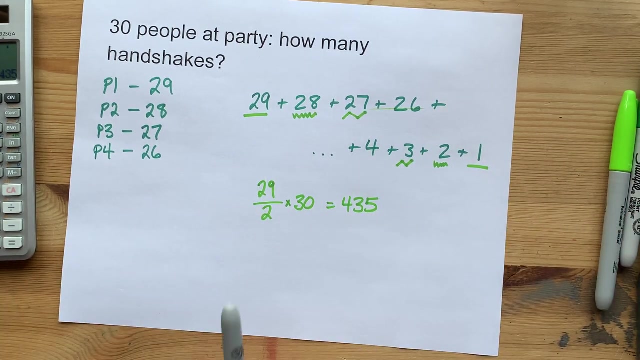 whatever, half of 29 is 14.5 pairs of 30 each. Cool, 29 times 30 divided by two, That gives me 435 handshakes. Nice, Again, you could have done all of this, adding all on your calculator. whatever, It's a free country There. 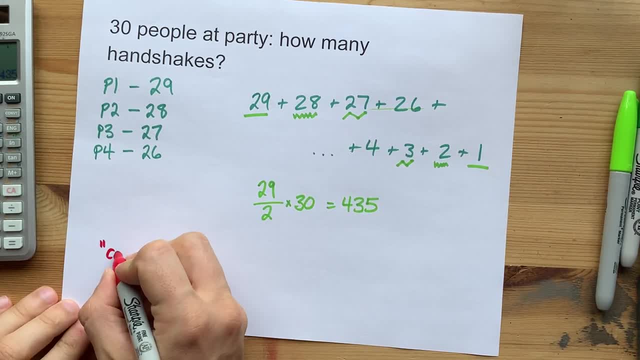 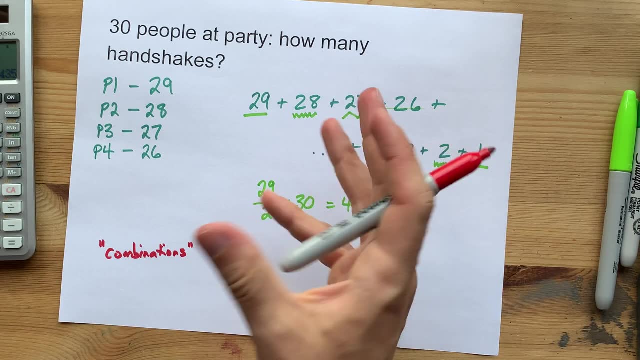 actually is one other way to do it. It is called combinations, And combinations is a very specific math term meaning arrangements or groups, So it's the order of things where the order doesn't matter, And what I mean by that is it doesn't. 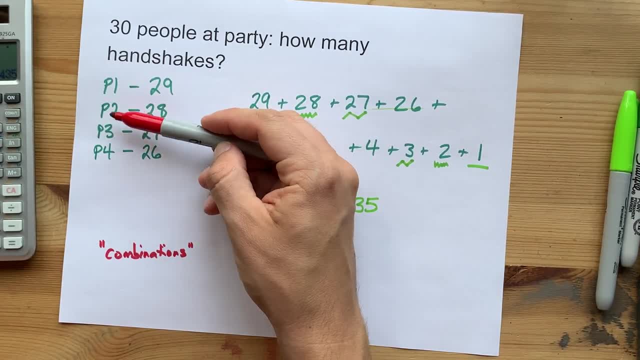 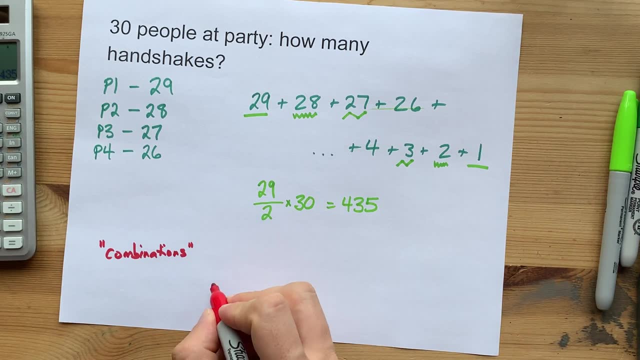 matter if person one shook person two's hand or person two shook person one's hand. Those are the same handshake. So you have 30 people and you are trying to figure out how many combinations you have of two each. Your calculator will do this for you And it's a little complicated of how it.